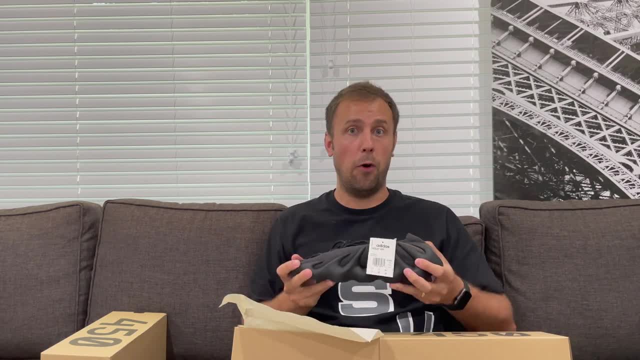 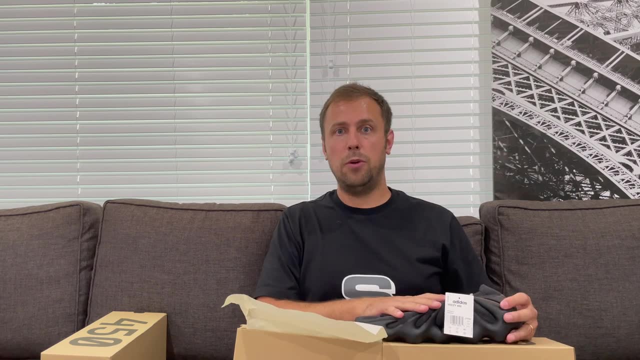 June 25th. Today is June 24th, so I was able to get them early. I had early access, again through Essence. I have two pairs in hand, a size 10 and a size 12, and, without further ado, let's get right. 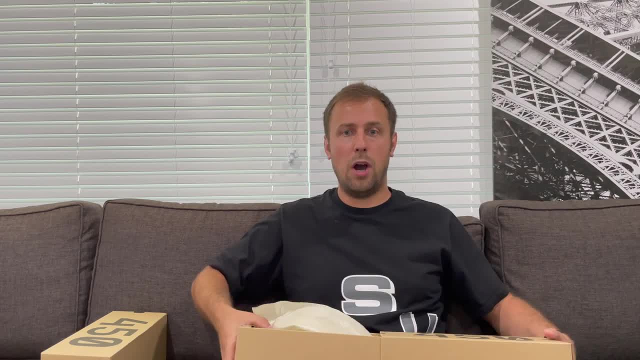 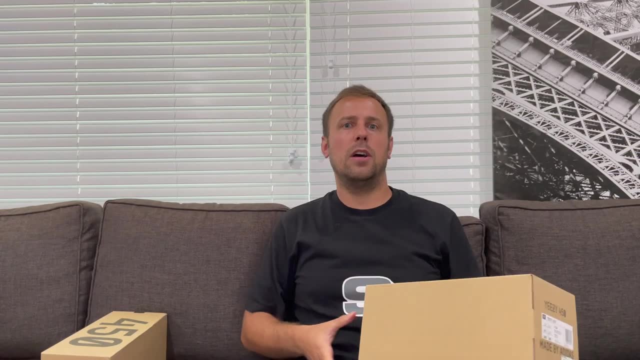 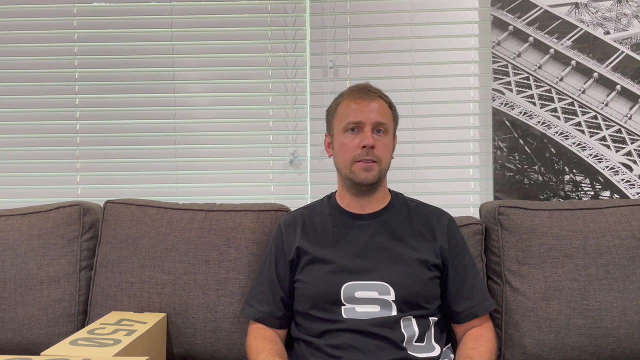 into it Talking, and looking at the box, it's the same with the previous one, the cloud whites. So that was the OG that came out in March. Retail- sorry. retail price it's $200 US and compared to the cloud white, the dark slate is. 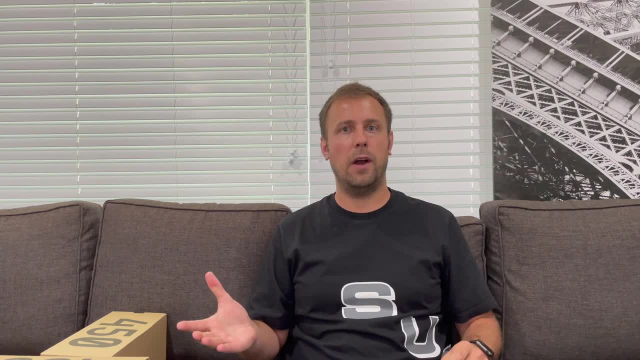 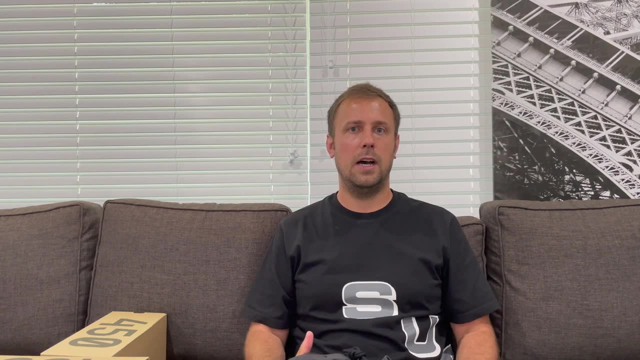 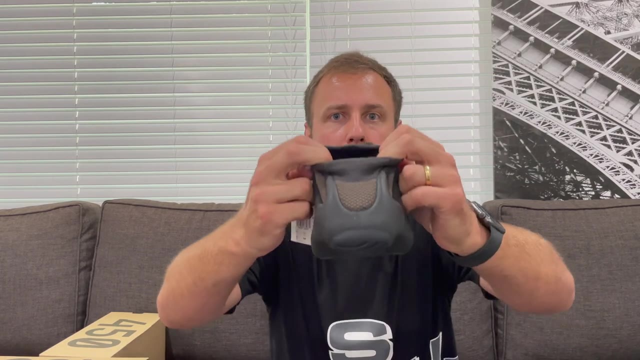 only coming out in men's sizes. The cloud white had infants and also kids sizing, but for the dark slate so far it only has men's sizes. So a couple of things that I've noticed. I haven't really looked at all the details, but on StockX you couldn't really 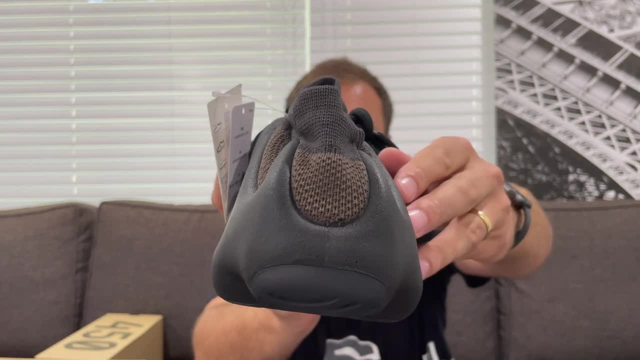 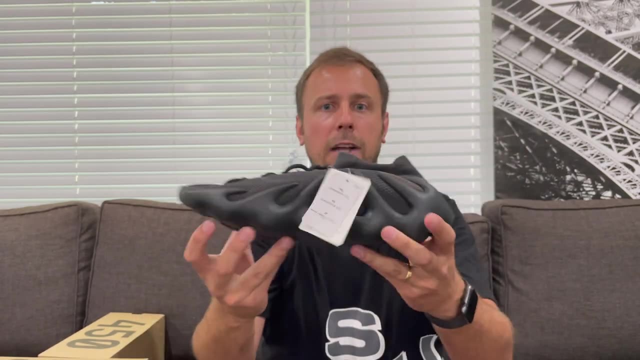 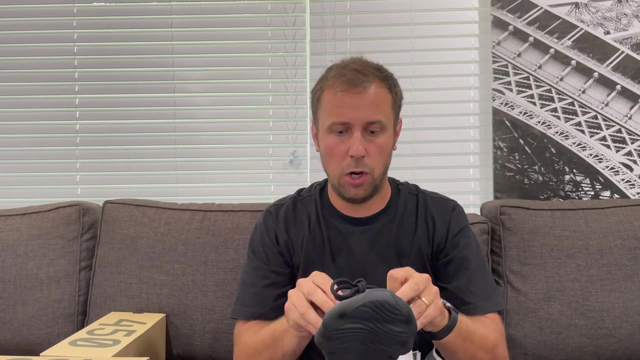 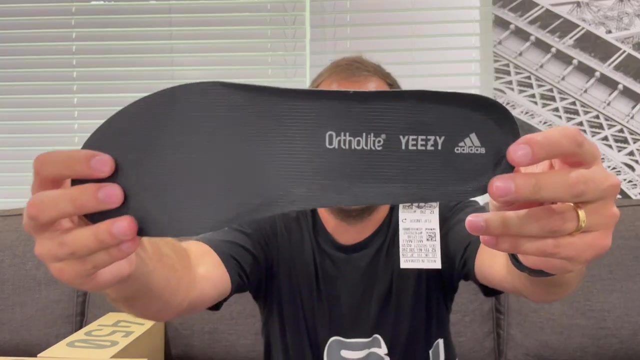 see on the pictures that this is actually a brown colorway on the on the back heel. It has like three stripes here, brown. Other than that the color is a really nice black. Same with the laces- No extra laces. The insole, it's the ortholite, so this time they went with. you know, comfortability And then 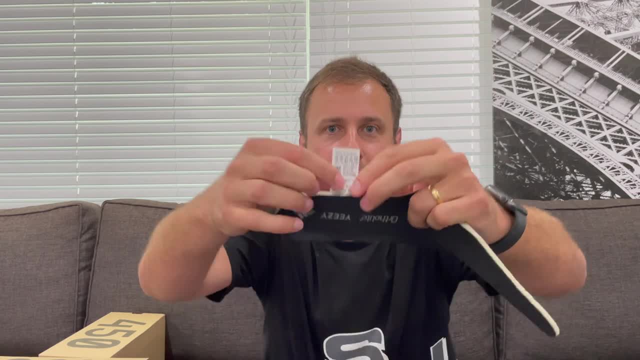 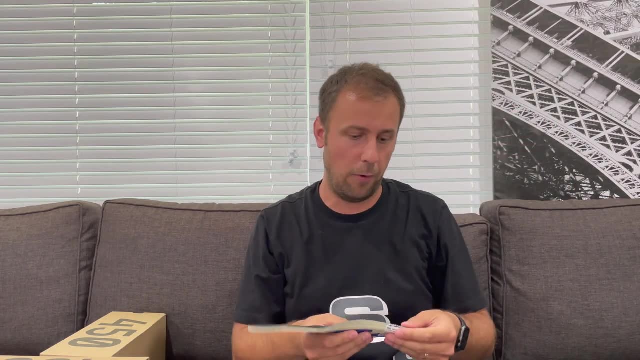 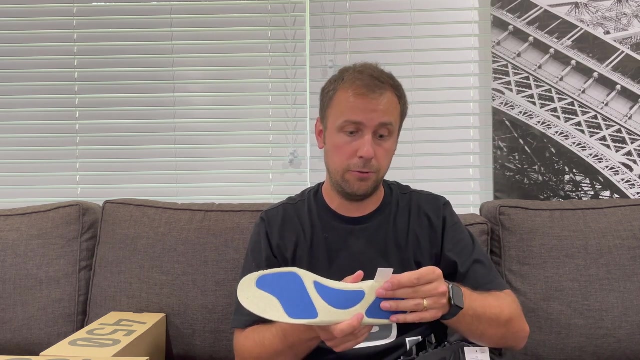 also interesting fact: if you look here on the tag on the side step, you can see that the laces are actually on the back. They actually tell you to flip under. So something cool that I haven't seen before. Also, what I've noticed is that this pair is made in Germany, So really interesting fact. 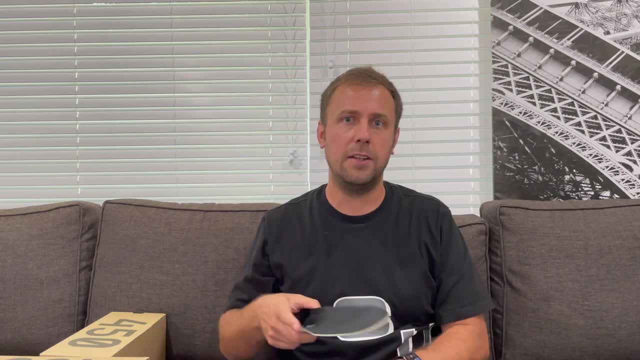 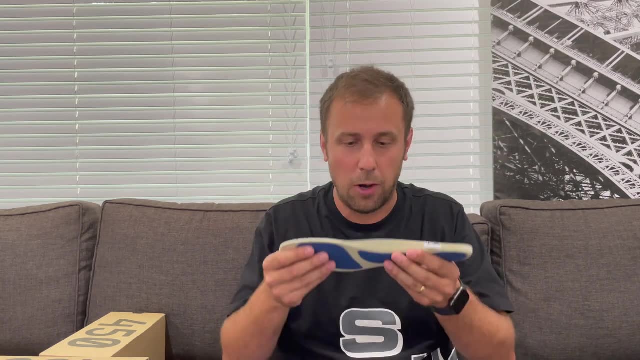 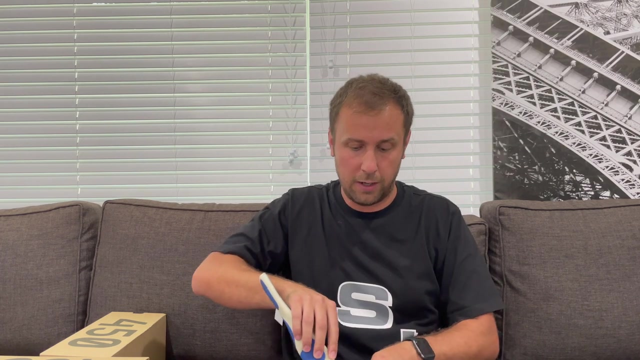 made in Germany. UK sizing- again, it's different than the US sizing. It's not like the foam runners and they actually smell really nice. So it's it's something like a chocolate. I want to say This is a really nice smell. As soon as I opened the box, I was really impressed with it In terms of sizing. 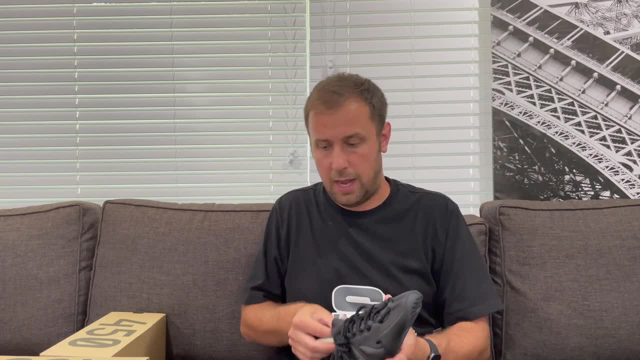 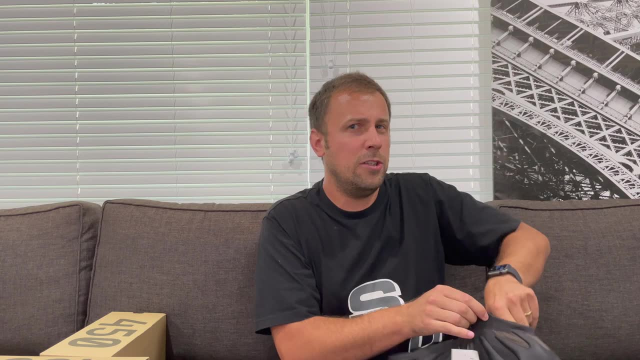 I'm usually at 10 or 10 and a half And I was okay when I put the size 10 when I tried it on. I'll show you guys some pictures. I was okay. I didn't really walk around, but it was. 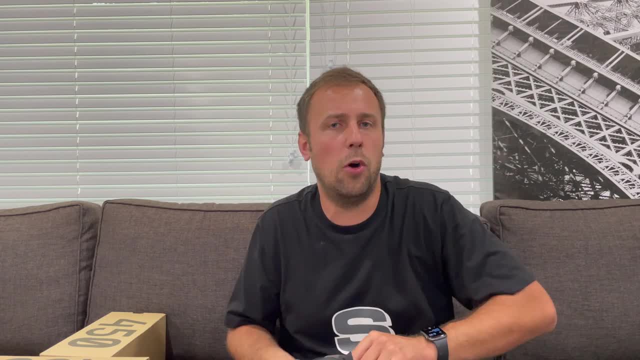 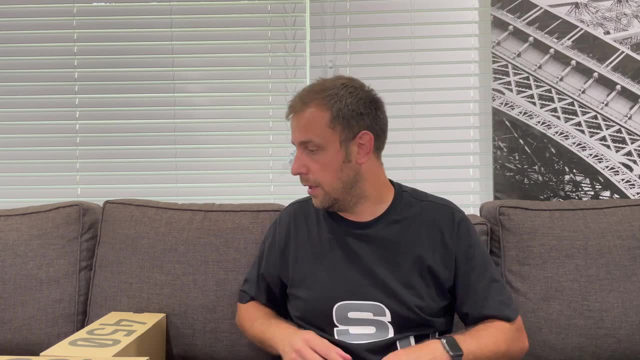 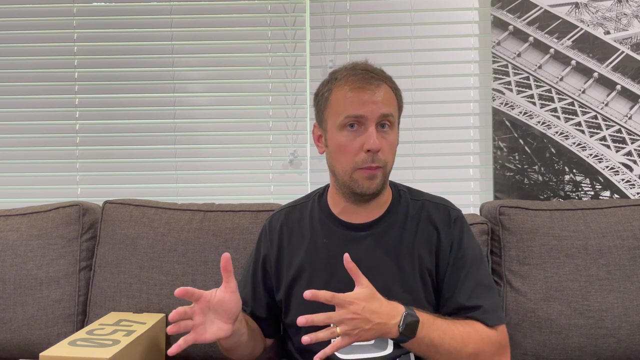 it was decent, I would say. So, if you want to go, maybe to the size, or if you have wide feet, maybe you want to go, you know, half a size up, Although, to be honest, I tried the, the size 12 as well. It was on the, on the bigger size for sure, But it wasn't uncomfortable. So you know, from 10, 10 and a. 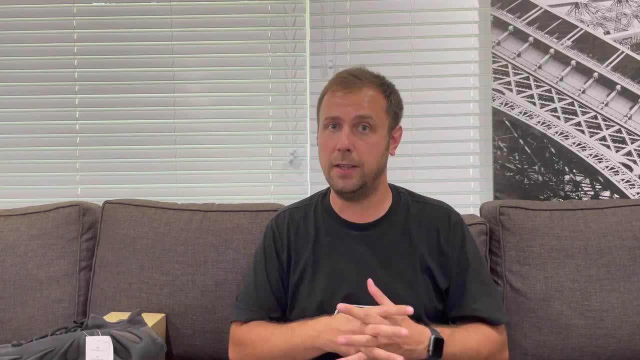 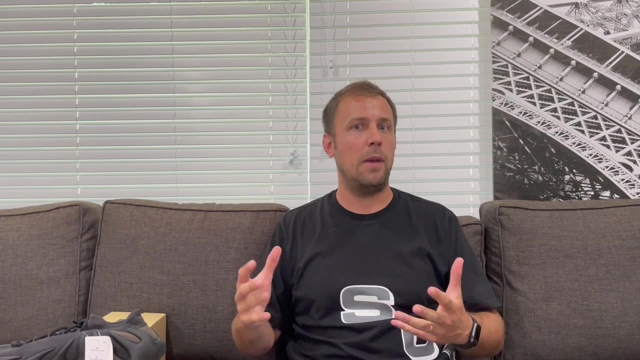 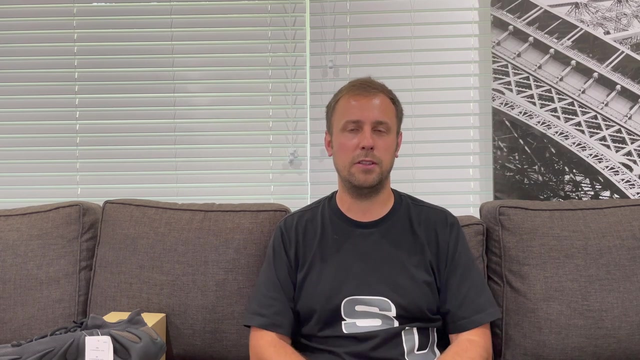 half to 12. it's quite a big difference, But I was okay with that, I am. you know. it felt good, Especially if you like your your shoes a bit loose. Maybe I would say again half a size up or one size if you really want to have that extra comfort or maybe extra space. Other than that, you know. 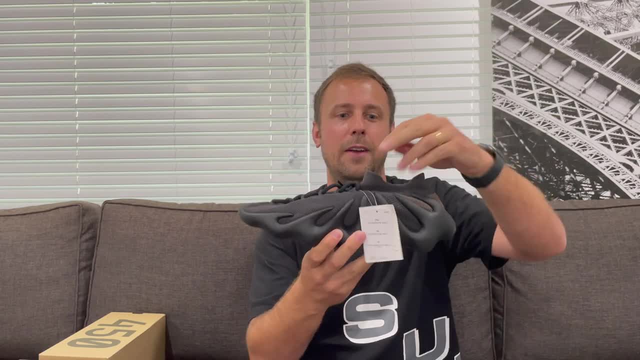 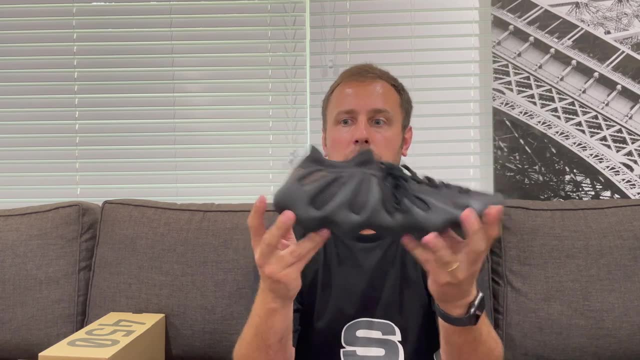 hard to say in terms of design, Because some people love it, some people hate it. Honestly, when I had the cloud white, I didn't really like them, But this being like an all black shoe with just a little bit of brown, I honestly like them. 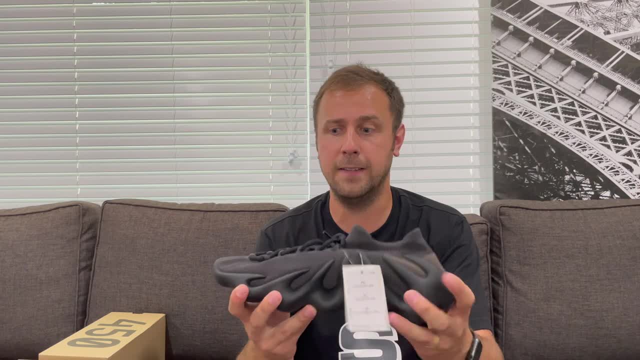 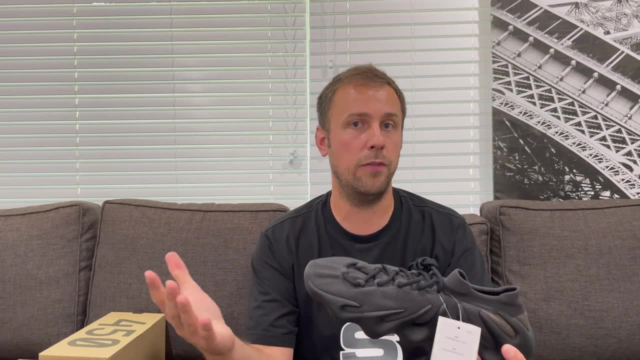 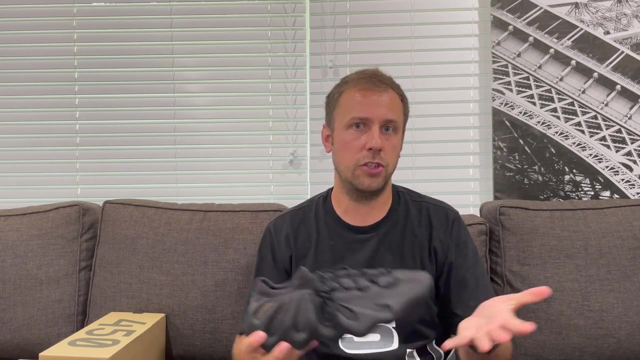 You know I was debating whether to keep a pair for personal or not. It's definitely a nice, you know, summer shoe, or all year round, if you know, if you don't have a lot of snow or a lot of rain. If you know, in your region- for me because I'm in BC, in British Columbia, Canada- we do get a lot of. 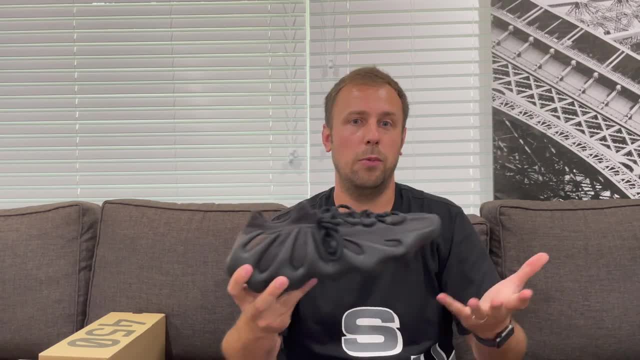 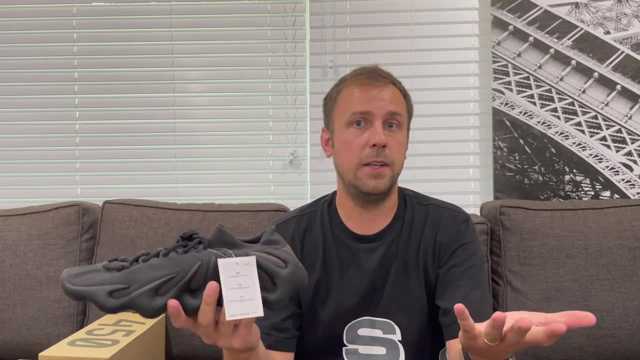 rain. So I could probably only wear this, you know, three, four months and that would be it, But nevertheless it's a really good shoe And, again, retail $200. it's close to, you know, the easy 350s. Those are $220.. So 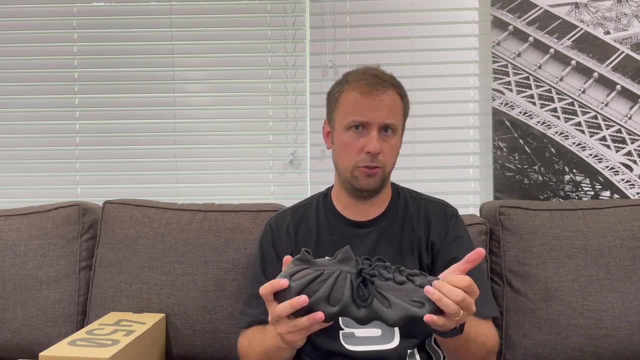 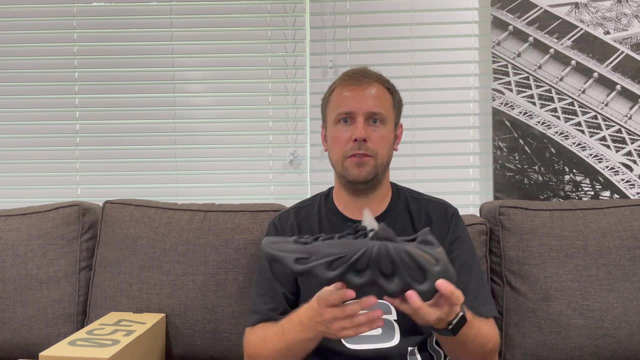 being made in Germany. I'm guessing quality control is really good on these Materials are really good. But that's about it in terms of the quick review. I just wanted to bring it to you. I'll show you guys a couple more pictures and I'll put a small- you know- rotation. one. Let's talk about resale. So right now, depending on sizes, these are going anywhere from $300 to $400 US. With me, I already pre-sold the size 12. I was actually able to sell it on goat. As soon as I had shipping confirmation, I went ahead and I listed it. And my payout is about $410, I believe, US dollars around there. Again, a better payout on goat compared to StockX. This is usually the case if you have early pairs, And not only. My suggestion would be, if you cannot pre-sell them locally, try and go for goats first and then maybe look at StockX. eBay might be another option. if you want to pre-sell them locally, Try and go for goats first and then maybe look at StockX. eBay might be another option. if you want to pre-sell them locally, Try and go for goats first and then maybe look at StockX. If you can pre-sell them as well, because I think for that you got like 30 days to sell them and you can probably get a better premium, even compared to goat For size 10. I've listed it, I haven't sold it yet. I might try local. but going back to resale depending on size, is anywhere? 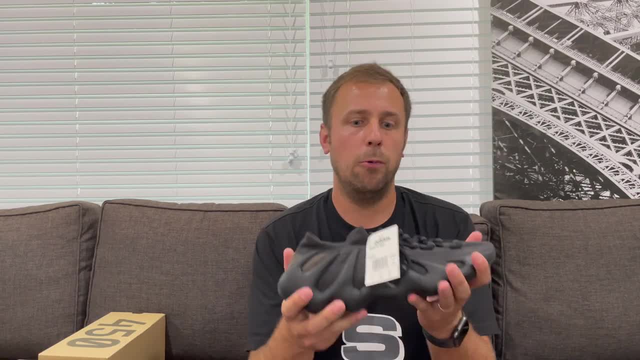 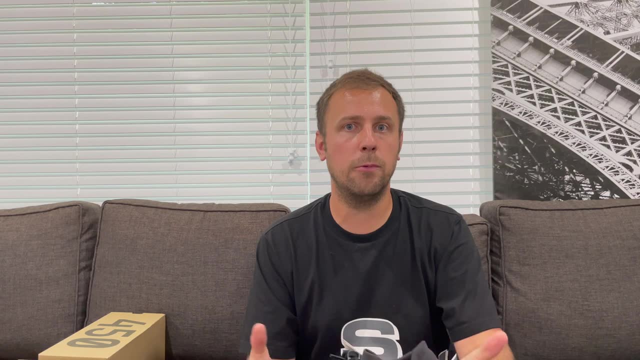 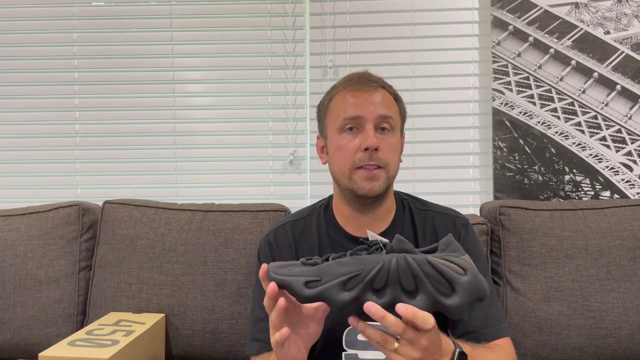 between $300 and $400 US. Will this go up? It's hard to say right now. I've said it over and over: the market is slowing down. we have so many releases coming, and then another factor you have to consider is you know the marketing behind the 450s, so i would expect to see a lot more of 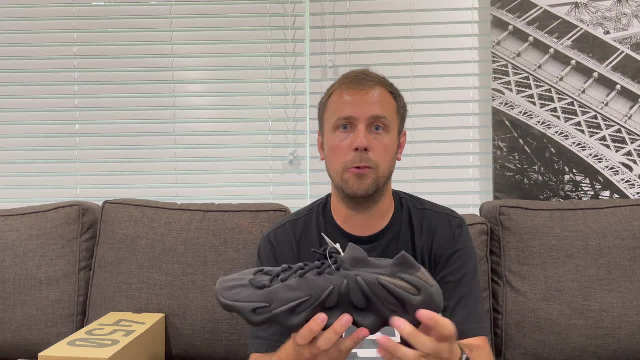 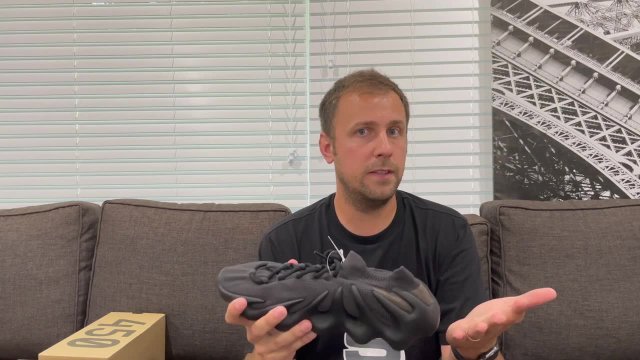 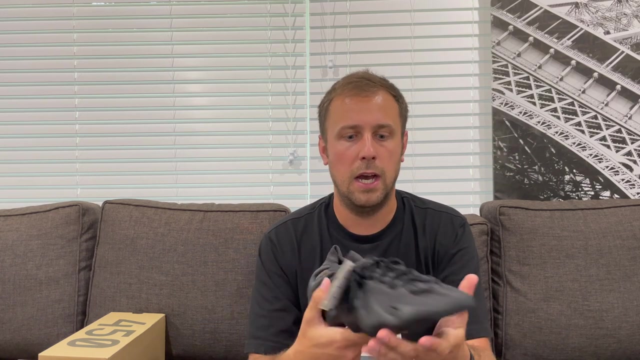 the 450s in the upcoming months, different colorways. so for that reason i would highly recommend that you guys sell them retail. it's not. it's not cheap, you know. it's two hundred dollars at the end of the day it's more than a jordan jordan one, um. but right now resale is looking really good. you can. 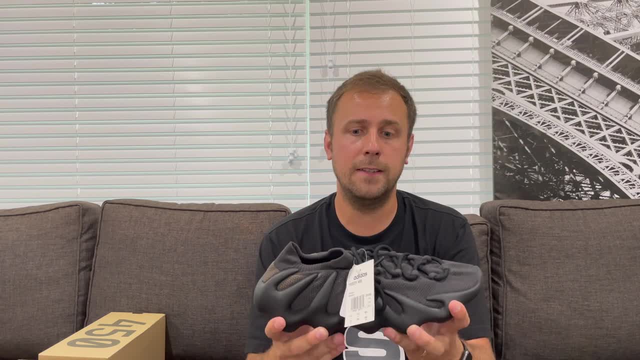 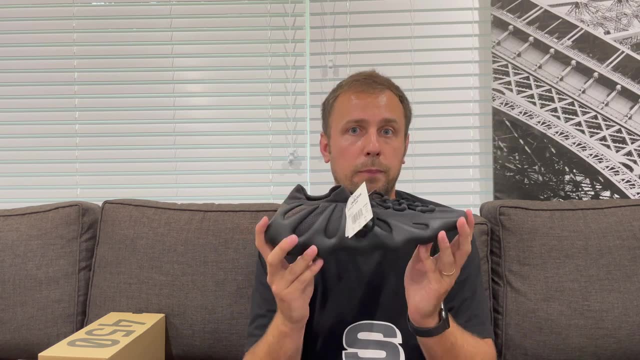 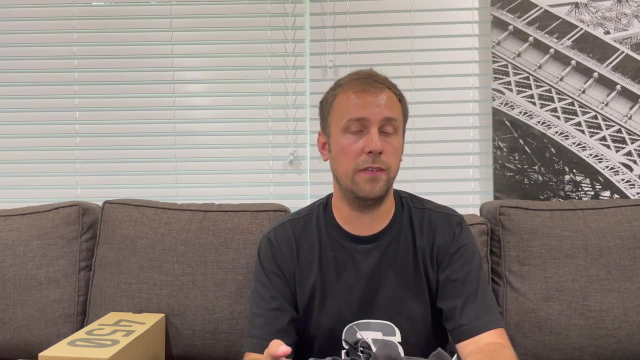 almost double your money, if not more than that, and you know if you look at other shoes and how much they're reselling, for this is a good profit. i would highly recommend that you sell them, unless you hit, like i don't know, 10, 20, 50 pairs, and then you might want to keep one or two. 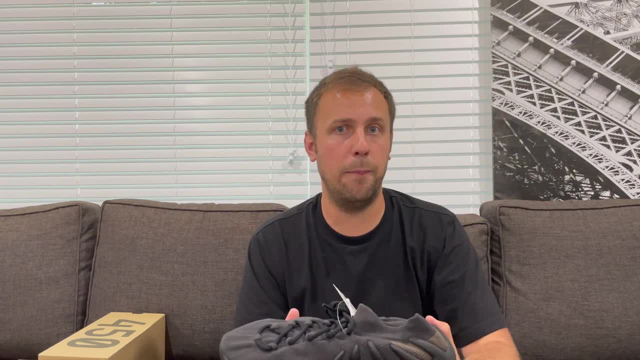 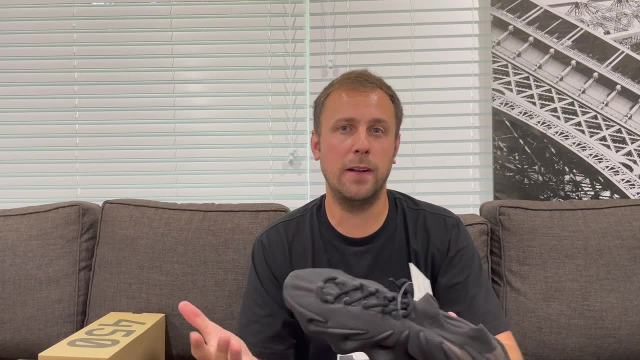 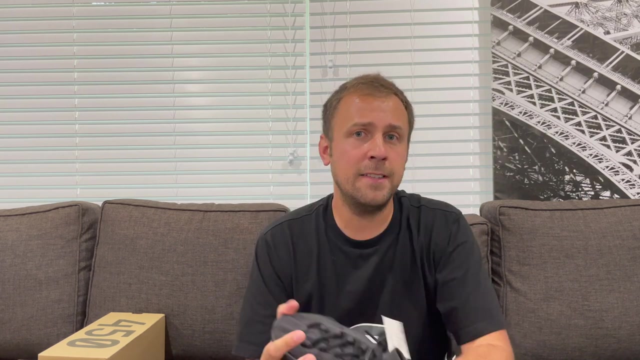 just in case you know it's gonna go, it's gonna go up in value. but if we look at the previous one, the cloud white, those have settled for i want to say around 500, if i'm correct. give or take depending on size. but that's the og colorway, right, it is a, you know, a lighter color, a better one for summer. 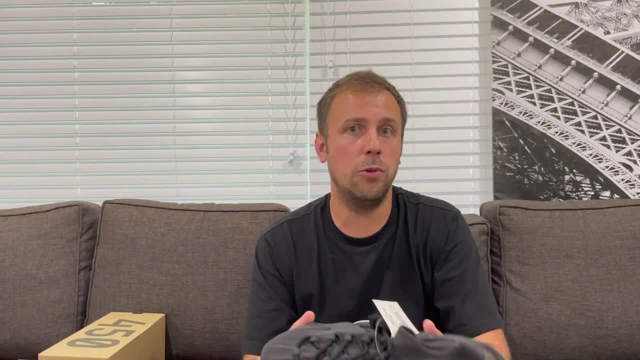 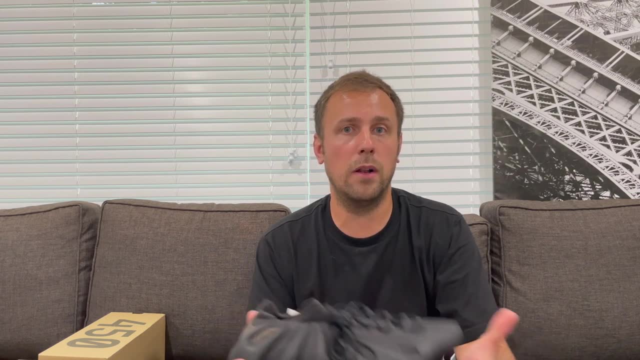 nothing against the all black one, but that's the og one. so this is like the second colorway that they're releasing and taking into consideration the overall the global resale market. right now i think 400 if you can get for resale it's a really good price. 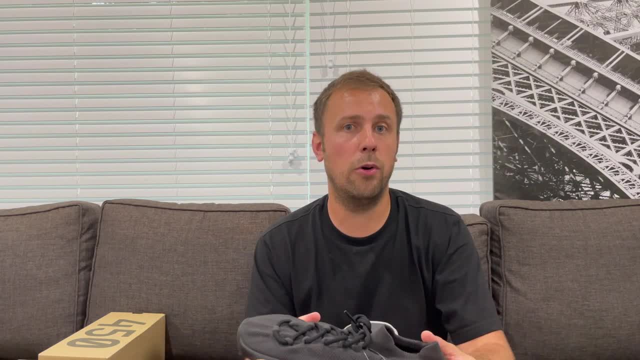 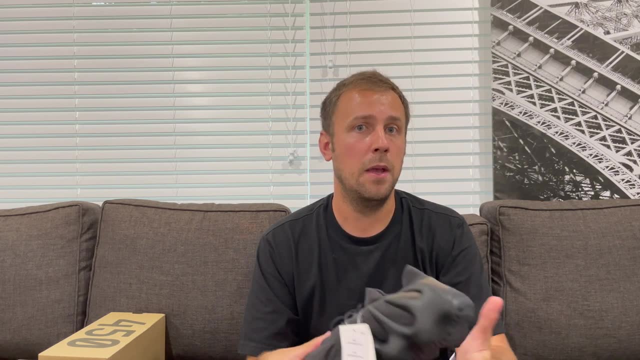 so if you have success tomorrow, on the 25th, or if you had access to early pairs, like i did, i would highly recommend that you sell them. but, as usual, let me know your thoughts. let me know in the comments down below: what do you think about this colorway? do you like it or not? i would highly. 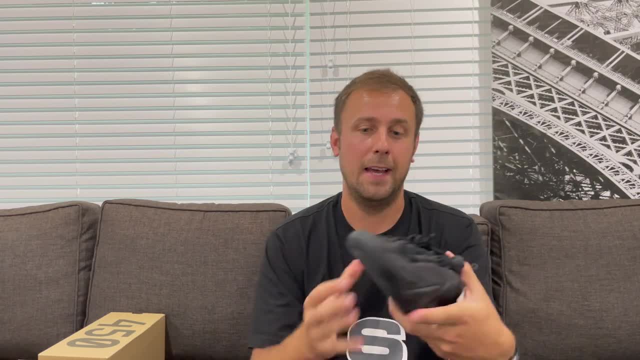 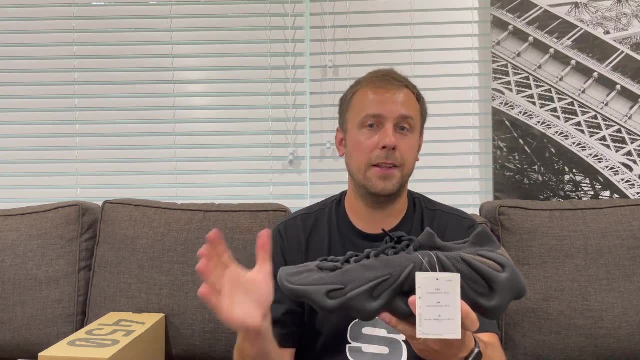 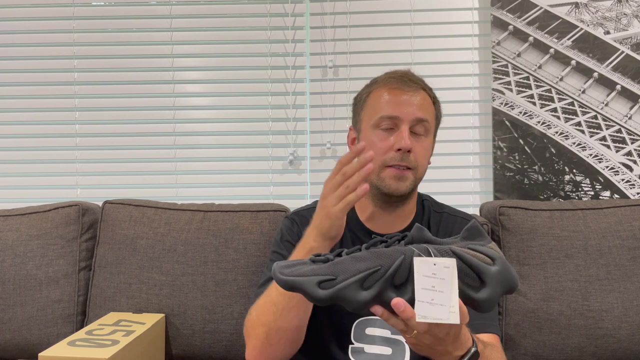 do you like it? um, are you gonna wear it? um, are you gonna resell it? are you gonna hold? what are your prediction? what are your thoughts? again, personally i didn't really like the first 450, the cloud white. but when i took this out of the box- and you know, made in germany, good quality.